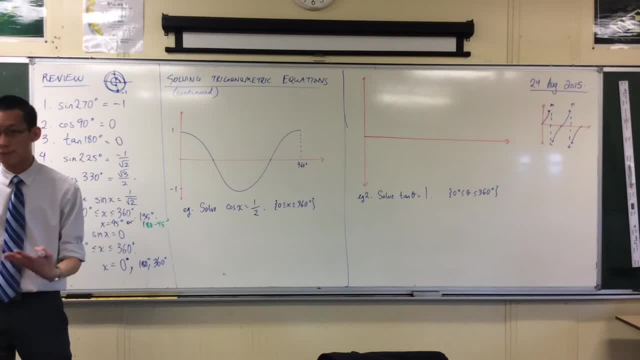 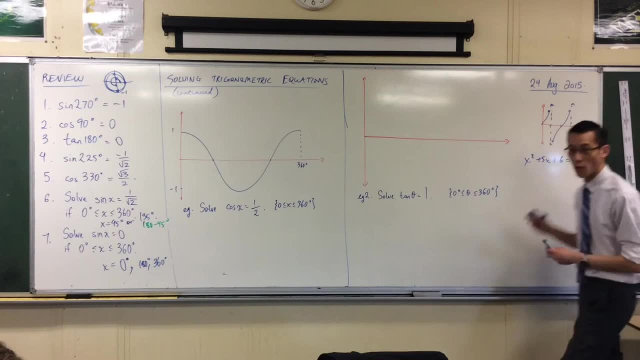 each of these really represents a graph. right, It represents a graph. So when I gave you this before, x squared plus 5x plus 6 equals 4,, for instance, x squared plus 5x plus 6 is a graph. it's a parabola, right, Like that? okay. 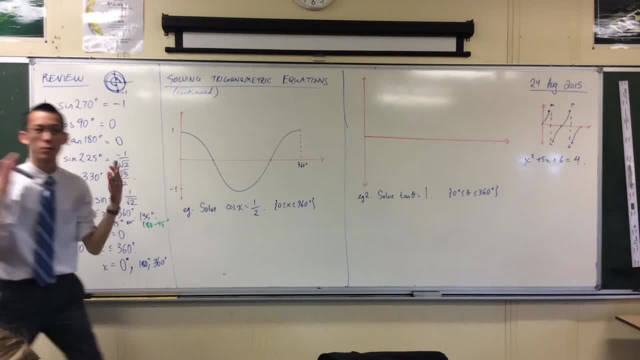 And 4 is also a graph. it's a straight line horizontally and I'm looking for where these two collide. okay, So cos x, there's my cosine. This is my cos x graph, right? What else should I put on here if I've got this on the right-hand side? 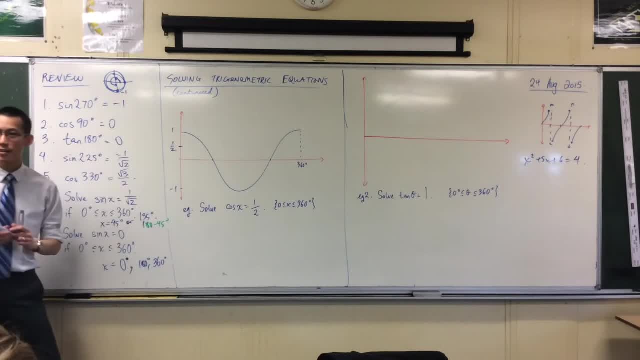 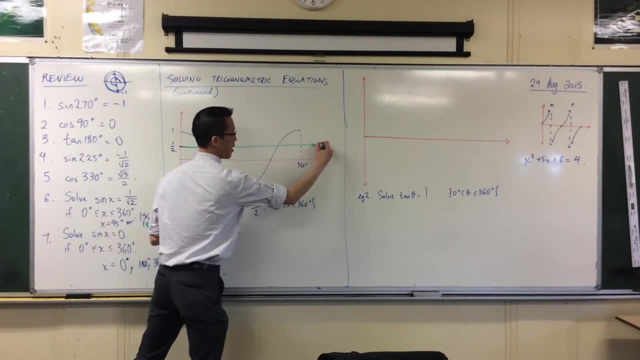 That's 1, right, So I've got a half there. So, right through the equation, through the graph, I'm going to draw in a half. Okay, That's a half, and my graph up here. the original one is cos x. 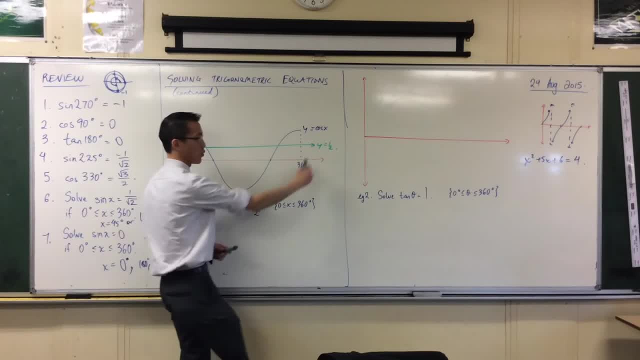 So if I want cos x equals a half, that's where cos x, cos x equals a half, And you can see I've got two points of intersection right: 1, 2.. Okay, So at this point you can see. 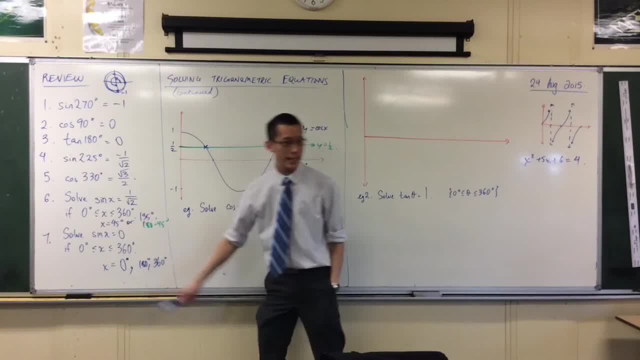 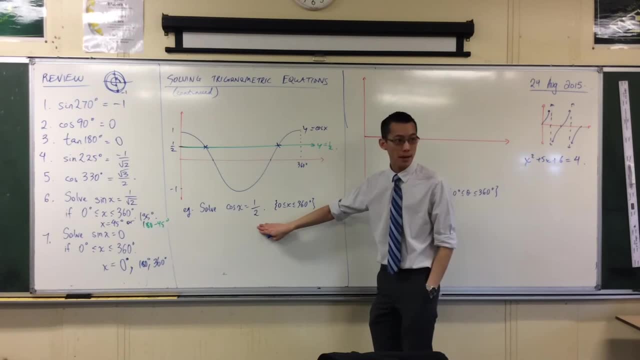 if we want the first solution, just like we did here and here, instead of sine inverse. I've got cos, So I should go cos inverse right, So shift cos If you pop in a half, okay, It should give you a solution which I hope you can start to recognise by now. 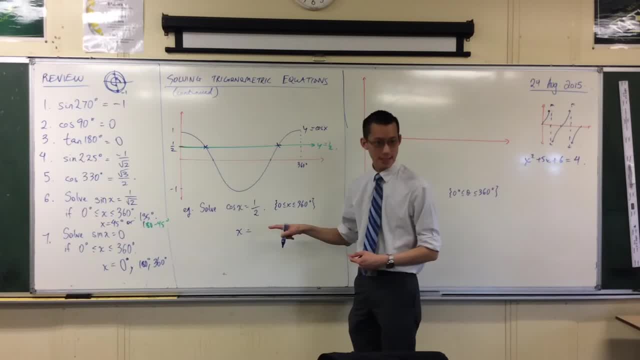 What's the exact value for cos that gives you a half. It's 60 degrees, isn't it 60 degrees? Now, just pause for a second. Does that make sense? Let's have a look at our cosine graph. I haven't finished it off yet. 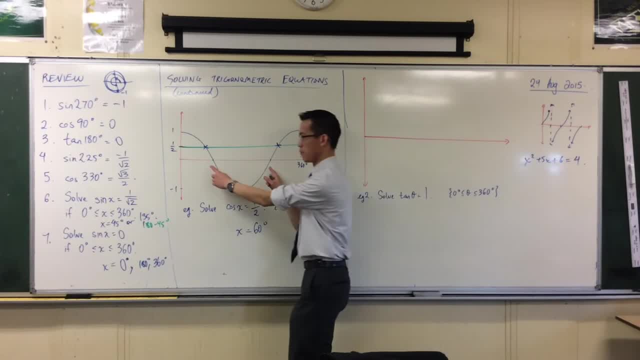 It's gone from 0 to 360.. But I haven't labelled all these important points here. For instance, what are these two guys? You actually know what? one of them is Cos 90, that's where it's equal to 0.. 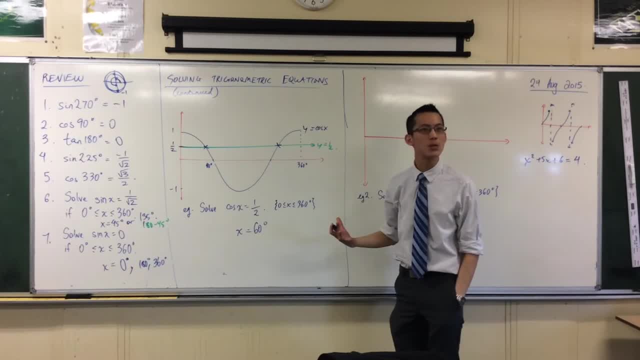 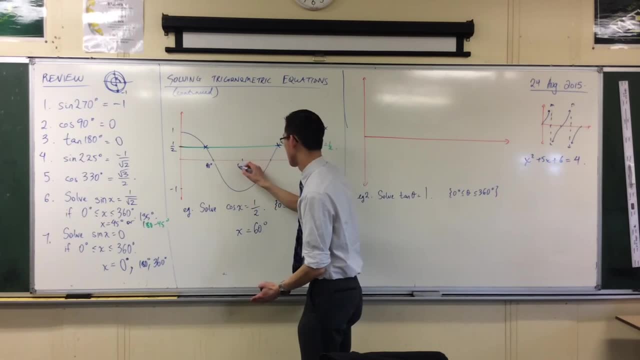 What's the other one? Have a look. What would you guess it looks like? Now I've gone all the way to 360 here, So halfway ought to be 180.. So that's where it sort of dips down. It has its valley right. 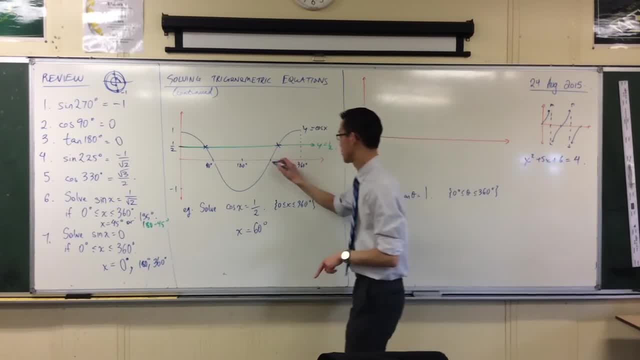 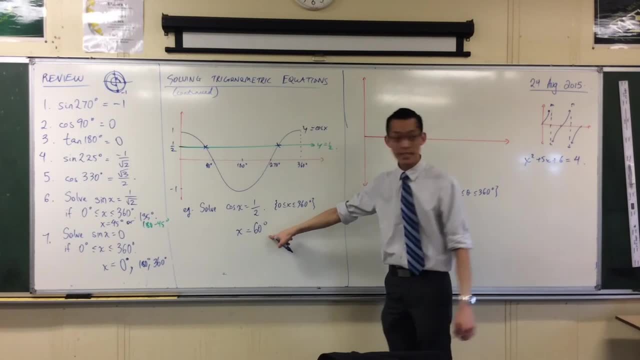 Which means the next one over will be 270.. 270. Okay, Now I have a sense of the scale of this thing. Does 60 degrees make sense? Does it look about right? I think so, Like. look at this.